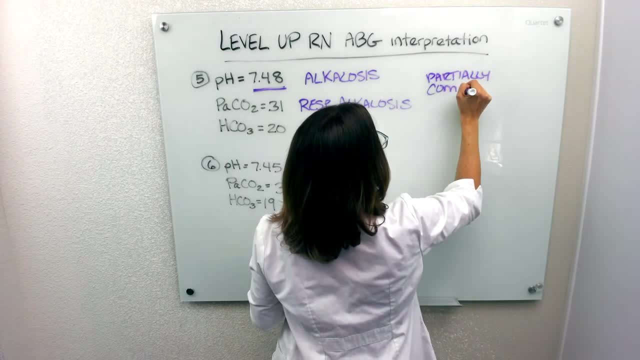 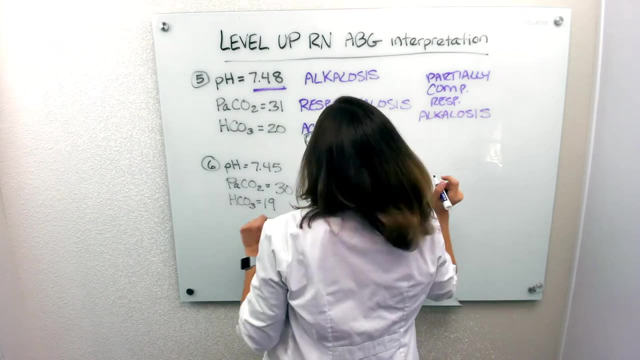 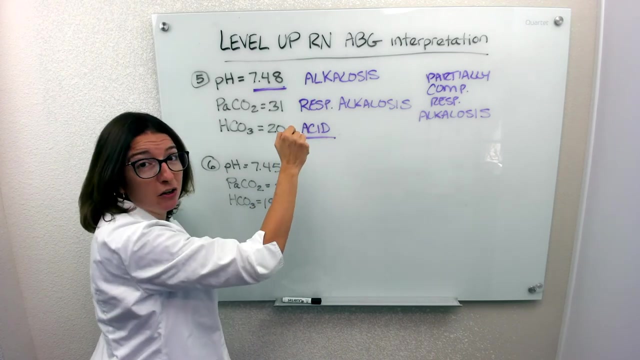 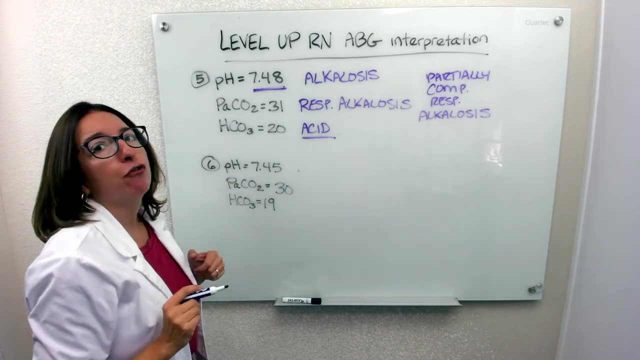 Partially compensated respiratory alkalosis. So flaming thanYeah Respiratory alkalosis. All right indicated that alkalosis. So again, the metabolic system is trying to compensate It's acidic, trying to compensate for the alkalosis, but it's not quite getting the job done. okay, Number six, pH is 7.45,. 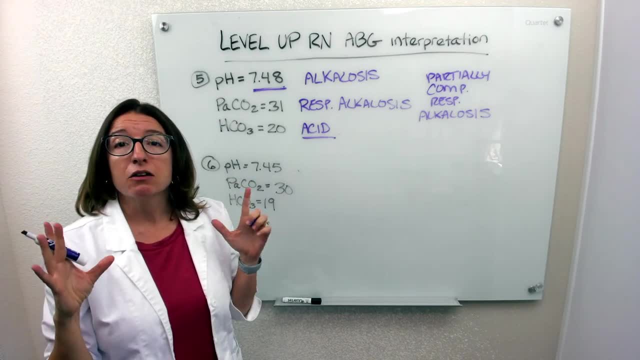 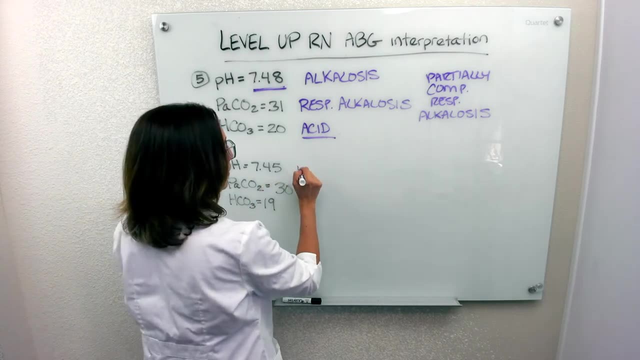 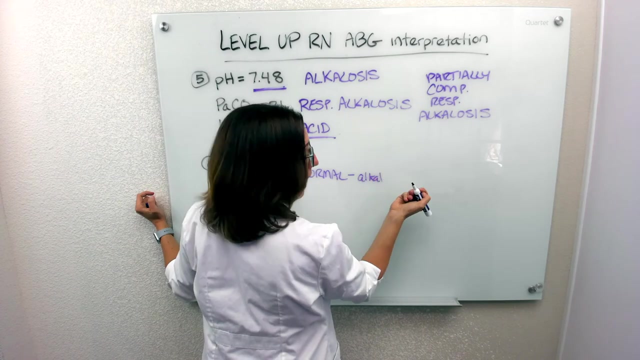 which we know is actually within range right, Because our range is 7.35 to 7.45, but it's kind of on the alkalosis side. So it's normal, but it's on the kind of alkalitic side, alkalosis side of things okay. 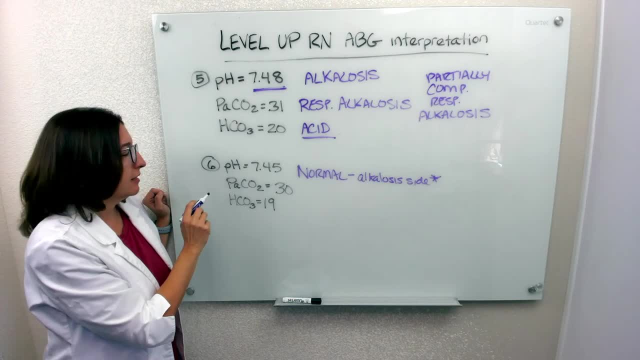 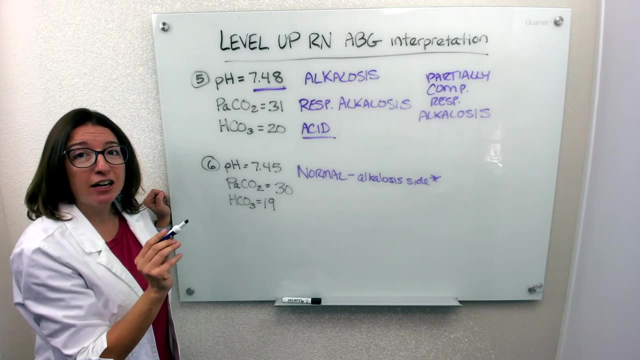 So let's see what's going on with the respiratory system and the metabolic system. So PaCO2 should be between 35 and 45.. 30 is out of range and it's out of range on the metabolic system Basic side. So we do have respiratory alkalosis going on. 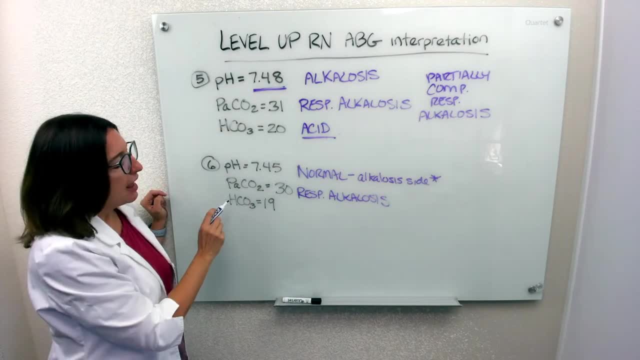 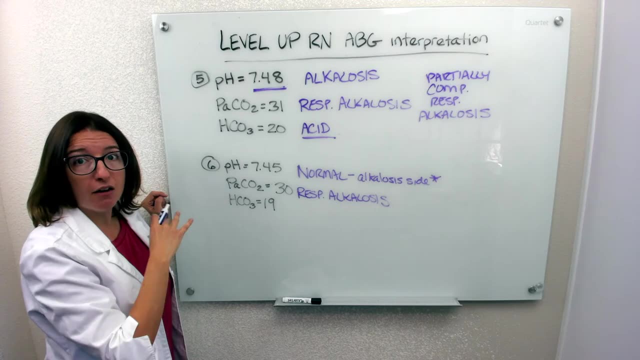 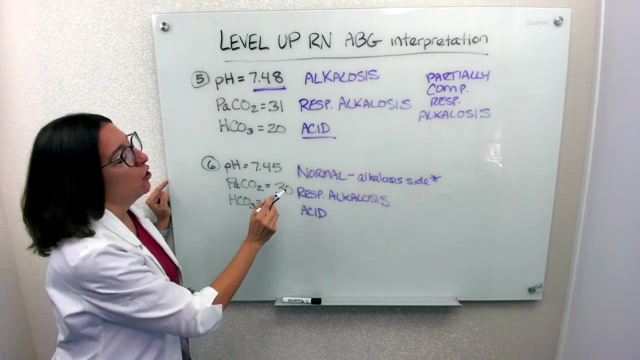 And let's see what the metabolic system is doing. HCO3 should be between 22 and 26.. It's 19,, which is on the low side, on the acidic side. So in this case we have respiratory alkalosis. that the metabolic system. 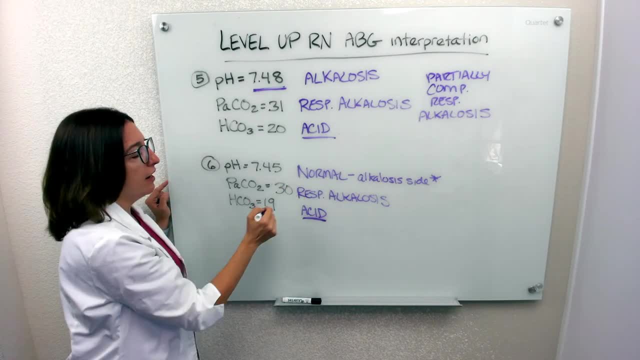 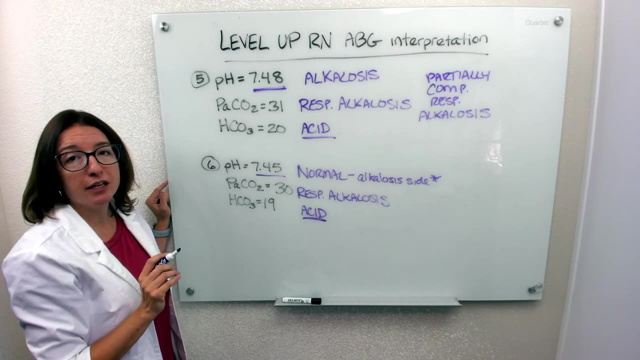 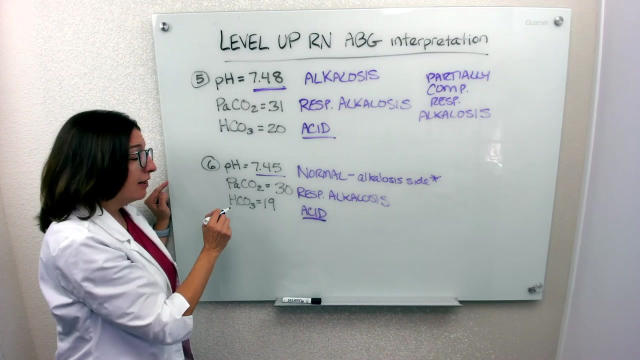 has compensated for and they were able to bring the pH up to a normal level. So we have fully compensated respiratory alkalosis in this case. So the respiratory system was acting out causing this alkalosis and the metabolic system came in, saved the day became more acid. 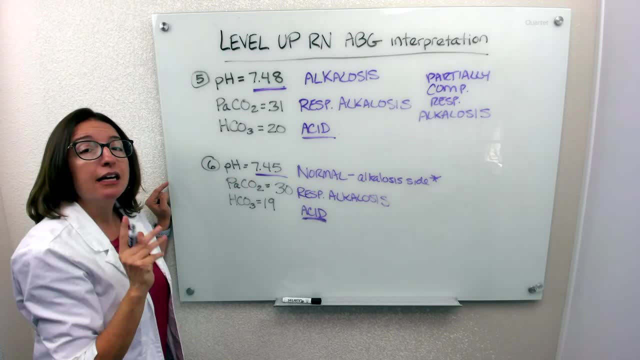 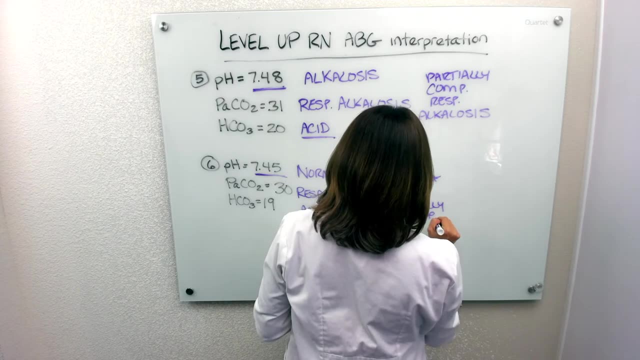 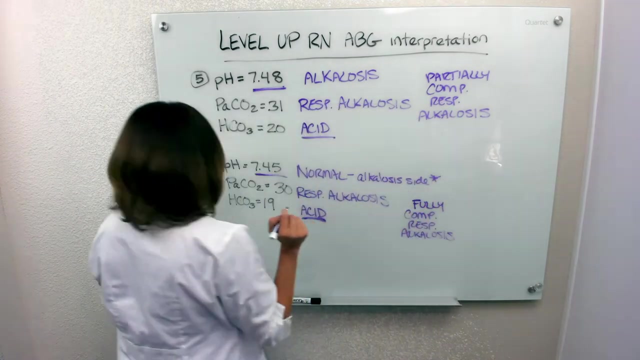 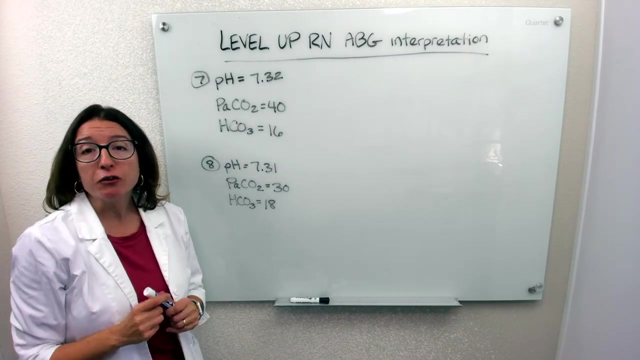 to help compensate for that and was able to bring that pH into normal range. So again, we have fully compensated. respiratory alkalosis: End of Lyme today, And that's problem 6.. Alright, number 7,, we have a pH of 7.32, which is out of range. right, Our range is 7.35 to 7.45. 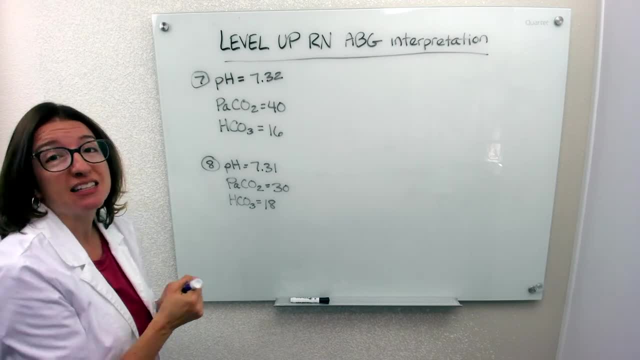 It's out of range on the low side so we know we have acidosis. So acidosis About 15 fogs every day. I Water them in the morning. I want to go out. This is really important for youradow mañana. 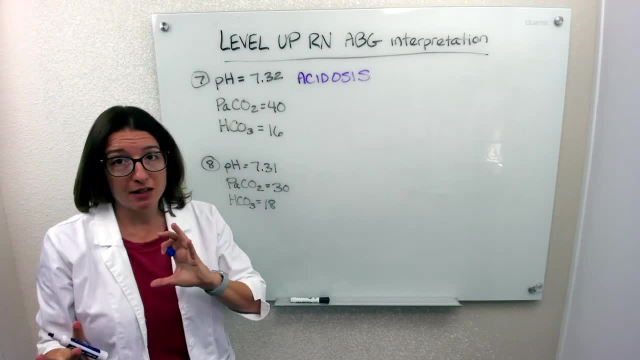 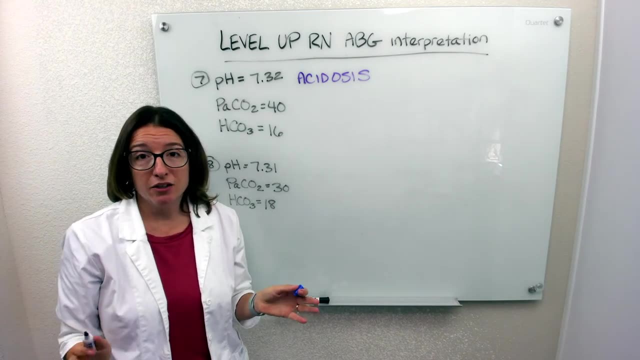 Now we need to see who to blame: the respiratory system or the metabolic system. Let's first look at the respiratory system. PaCO2 is 40, which is in the normal range, because our normal range is 35 to 45. So we have normal respiratory. 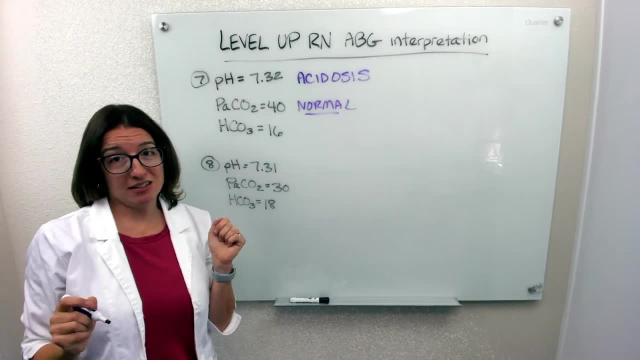 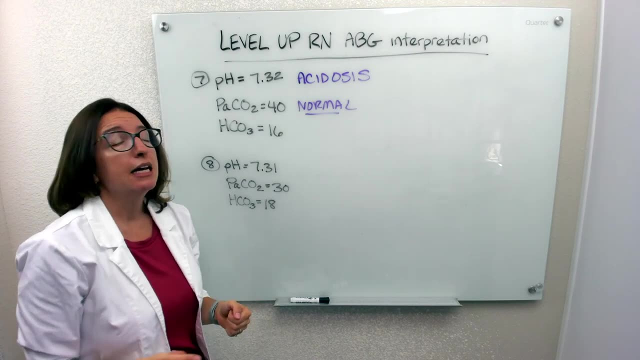 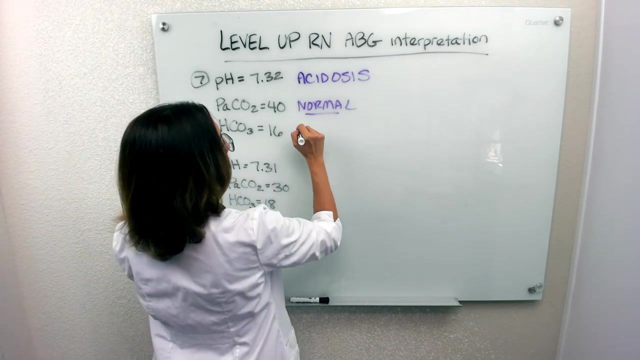 So we know this is not causing the acidosis. So let's go down here to HCO3 or the metabolic system Should be between 22 and 26. It is out of range on the low side, so it is causing the acidosis. So we have acidosis and it is caused by the metabolic system, So we have metabolic. 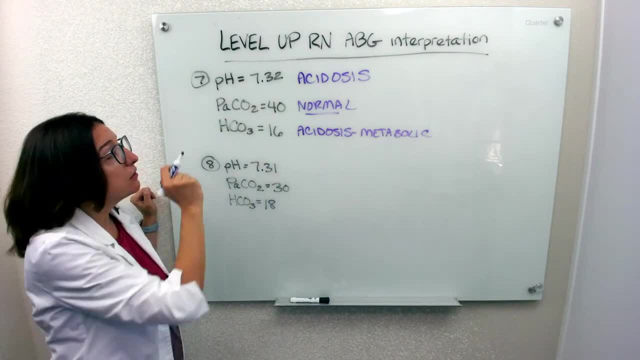 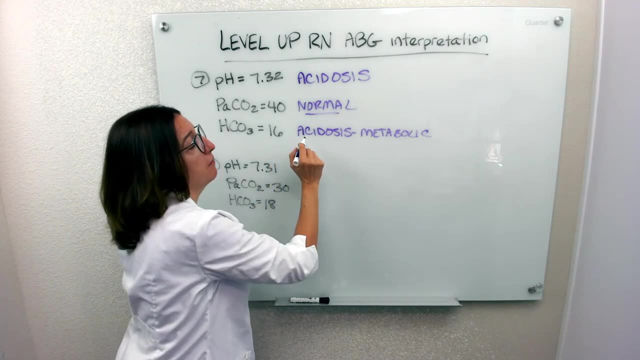 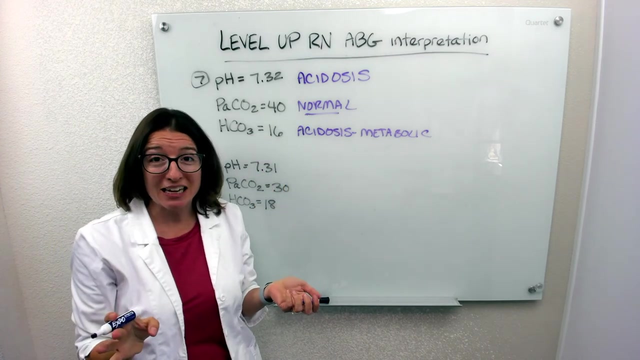 acidosis. Is it compensated? Is the respiratory system trying to compensate for the issue that the metabolic system is caused with metabolic acidosis? No, It's just chilling out in its normal range. right, It's 40. It's not trying to do anything. 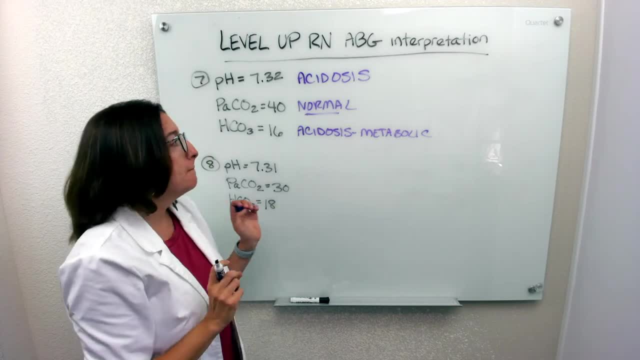 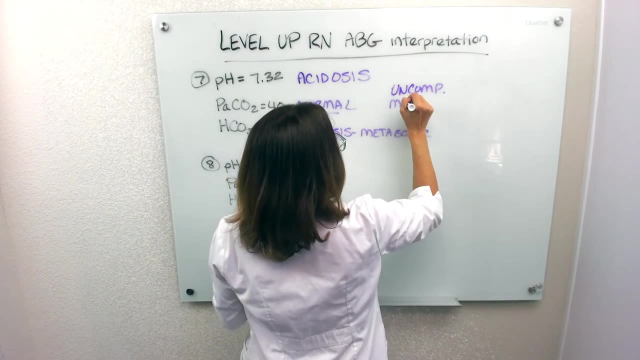 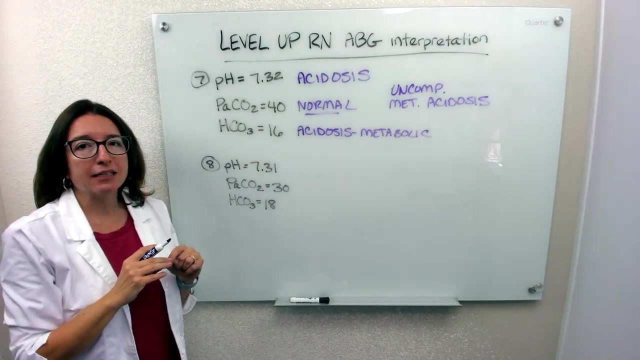 So in this case we have uncompensated metabolic acidosis, Uncompensated metabolic acidosis. All right, Let's do problem eight together. pH is 7.31.. So again, it's out of range on the low side. 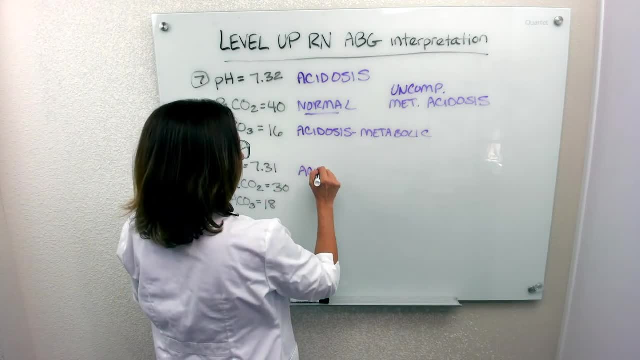 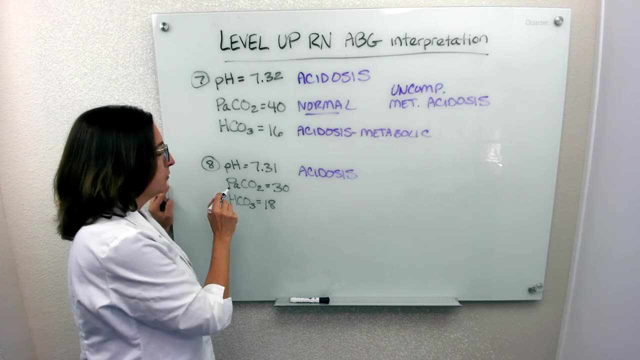 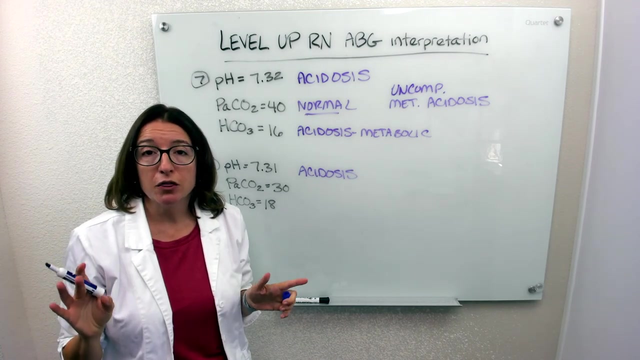 So again, we have a metabolic system, So we have a metabolic system. So we have a metabolic system, So we have acidosis. Let's see who to blame. All right, so step two: Look at the respiratory system. PaCO2 is 30, which is out of range. right, The range should be between 35 and 45.. 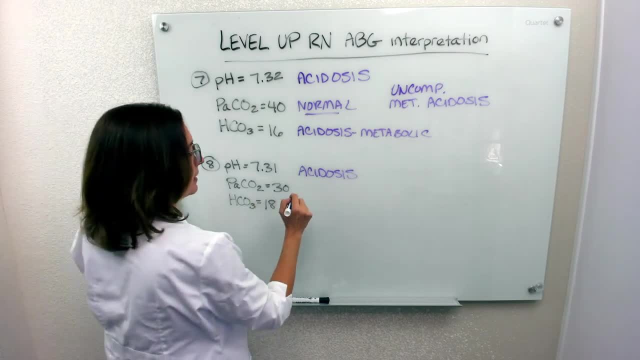 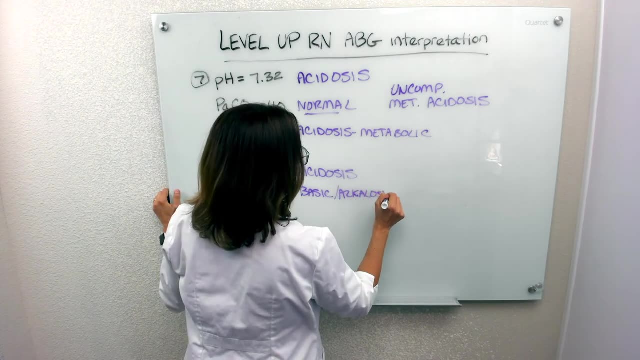 It's out of range on the low side, so it is basic, or you could say alkalosis, Those are kind of interchangeable. Now this is a very common, This is a very common mineral. This is a very common mineral. This is a very common mineral. So it is very common. So it is very common. This is a very